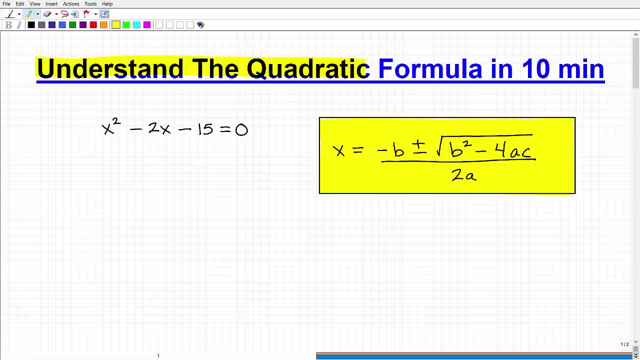 Okay, so in this video we want to understand the quadratic formula. Let's see if we can do it in about 10 minutes or so. Now just some kind of context about this formula and the subject that it relates to. Basically, we're going to be studying the quadratic formula in Algebra 1.. 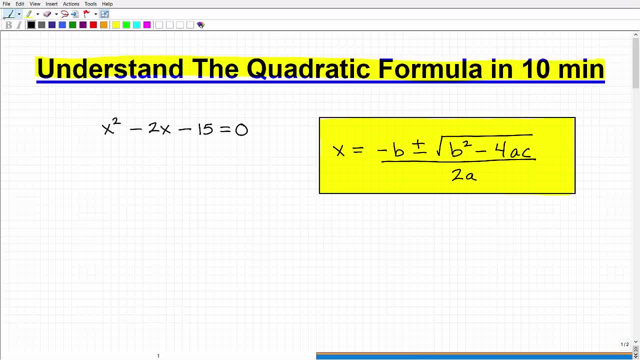 You may see it a little bit in pre-algebra, but it is an absolutely critical formula for you to know. Okay, so let's just give you some background real quick on why you need to know it, and then we'll get into the actual formula here. 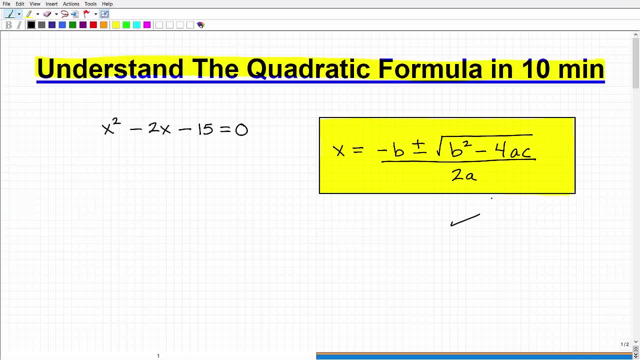 So, just real quick, there's the actual formula. So if that looks familiar to you and you want to know how to basically apply it, just be patient and we'll get there in one second. All right now. what we have here is an example problem that we're going to do. 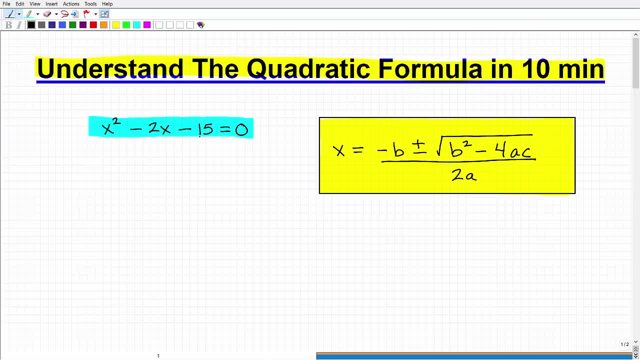 Now, this is a polynomial equation. Okay, it's a polynomial, Very specifically a polynomial. I'm just going to abbreviate Now. you study this in algebra, but polynomials specifically have a special characteristics about them. Okay, if you look at this polynomial, its highest power is 2.. 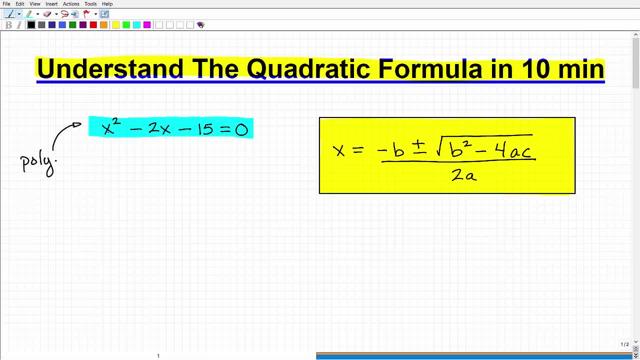 It's a second-degree polynomial. So, by definition, when you have a second-degree polynomial, it's what we refer to as quadratic. Now what's important about that? Well, this formula here only applies to quadratic equations. So we're trying to solve this quadratic equation. 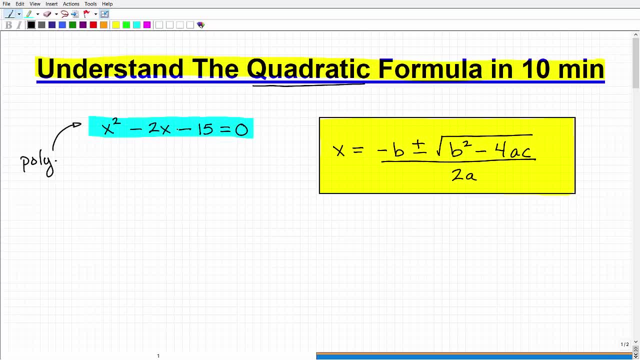 and there's various ways that we can approach it. Okay, so the first way that you would want to try to approach this particular problem is to solve it by factoring. Okay, it's always the easiest way to do that. As a matter of fact, this particular polynomial equation can be factored. 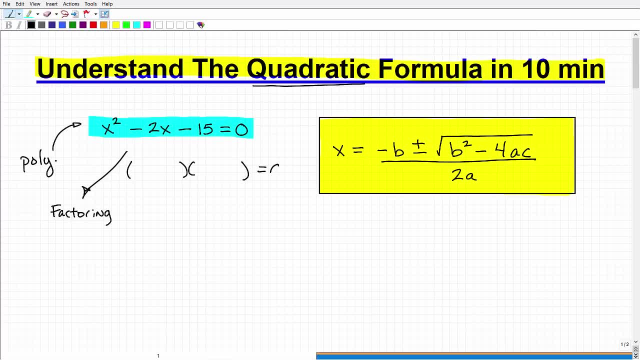 In other words, you can factor. you can factor this trinomial: okay, set it equal to zero, just like this, and then you would go ahead and set each of these factors equal to zero, and then you would solve. So I don't want to. 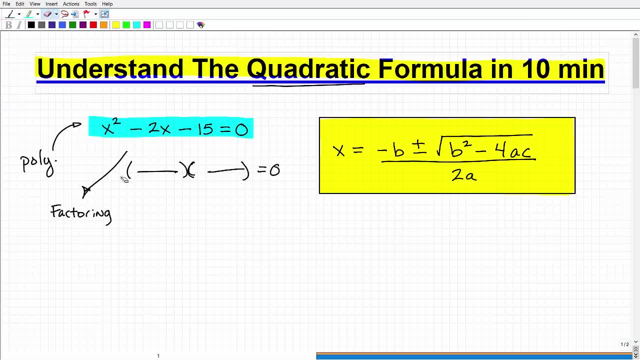 I'm not going to get into this too much more in this particular video, because this video is about the quadratic formula, but I'm just telling you in general, when you have a polynomial equation, you always really want to try to use a factoring technique to solve it. 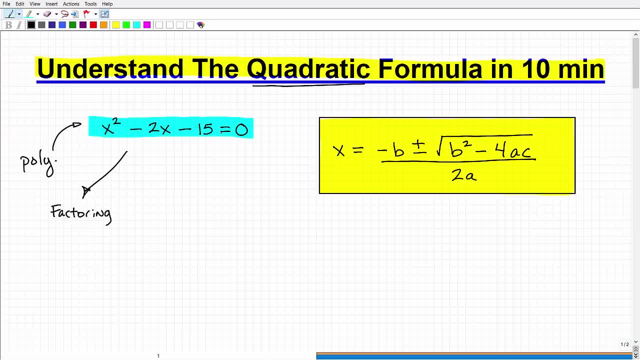 Now there are polynomials that cannot be factored, and that is where the quadratic formula comes into play. okay, Because a theory about polynomials is the following: okay, This second-degree polynomial or a polynomial to the highest power of two? okay, 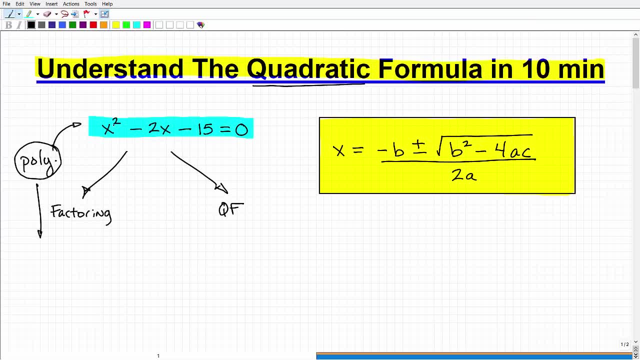 There's a theory that says the following: Whatever your highest power is of a polynomial equation, that's how many solutions you have. So this little guy here, this being the highest power of this equation means and it's x squared. so I'm looking at that little 2 there. 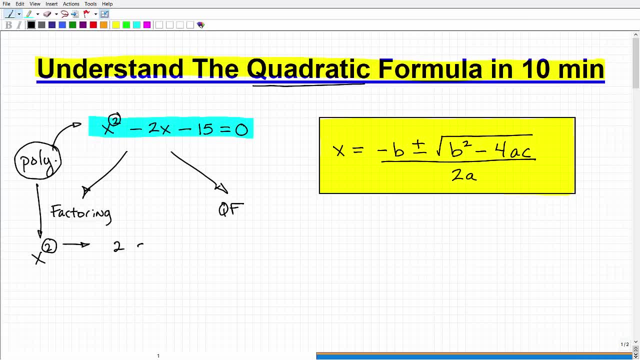 that means that this equation has two solutions. It has two solutions Now, oftentimes the solutions, the name for solutions- sometimes we refer to those as zeros and sometimes roots- okay, So they're kind of semi-interchangeable terms: a root, a zero, a solution. 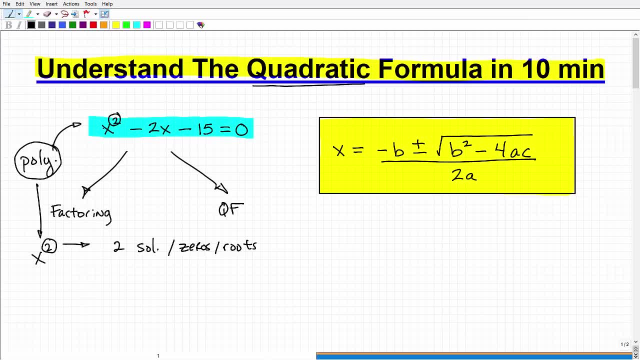 But basically they're going to be the solutions to an equation when you have a polynomial set equal to zero. okay, So you need to really kind of strengthen your understanding of polynomials in general and you know basically what they mean and what the kind of characteristics about them. 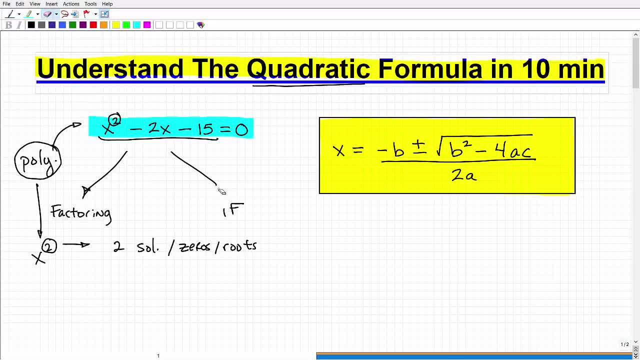 in order to really successfully apply the quadratic formula. You just don't want to be throwing any polynomial into the quadratic formula because you know it's a special needs tool. let's just say, okay, We use it when we need to use it. 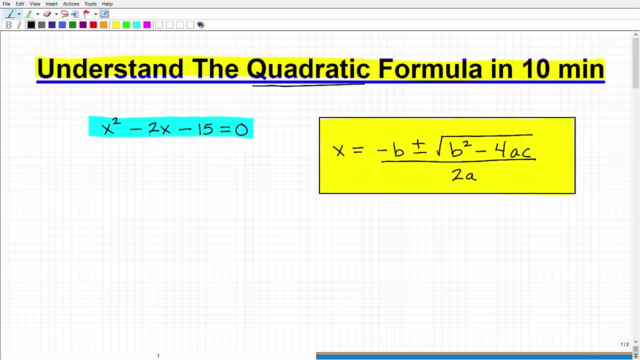 All right. so here we have a polynomial equation, quadratic equation, degree 2 polynomial. And the way we're going to go ahead and approach this problem using a quadratic formula is: first, we want to write this in what we call standard form. 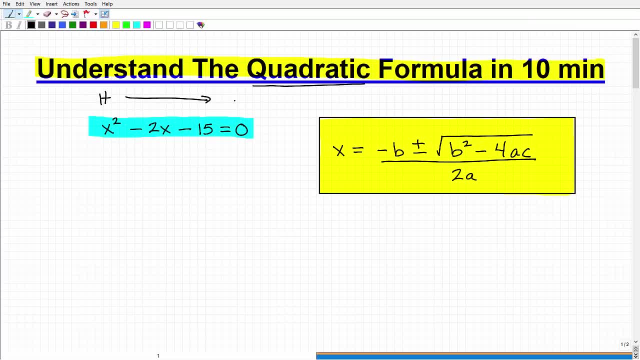 And that means it's from the highest power to the lowest power, And that's generally a number. So here you can see that this already is written in that form. We have f, We have x to the second And then we have an x term. 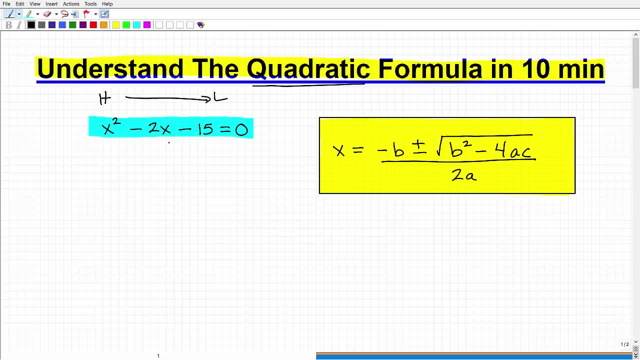 And then we have a number And it's always going to be set equal to zero. So if your polynomial is not written in this particular form, you need to kind of shuffle things around such that it's in this form. This form is called standard form. 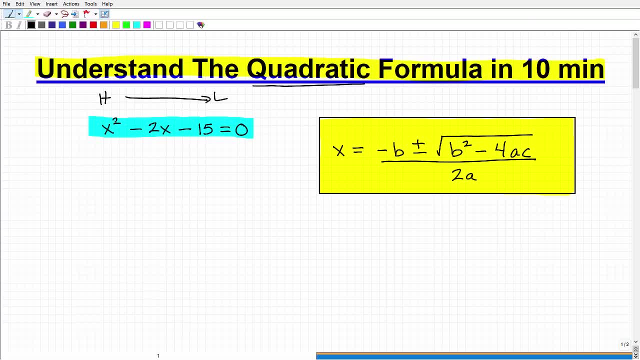 Highest power to lowest power. okay, So it's going to be degree 2, degree 1, number equals to zero. Okay now, once you have that, and then we can go ahead and actually start plugging some values in. 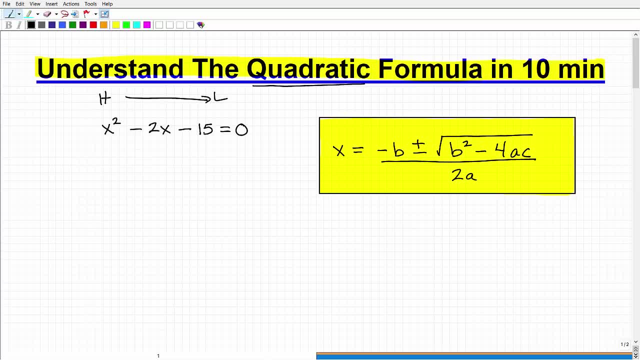 Now let's go ahead and look at some coefficients of this polynomial. So x squared is actually technically a 1 there. This is 1x squared minus 2x minus 15.. So this guy we're going to give a specific 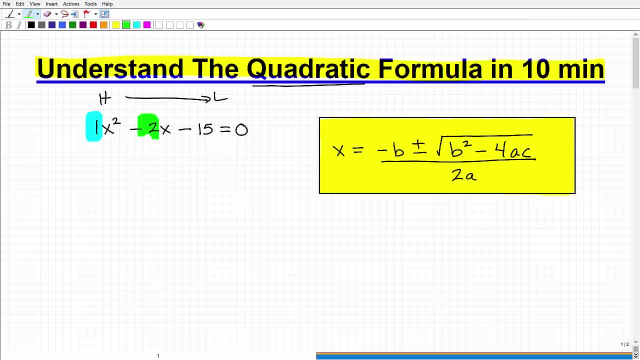 assign a specific variable to And this guy here And this one over here. Okay, So the number in front of the x squared in the equation is a. Okay, So this is a is equal to 1.. All right, This. the number in front of the x term is b. 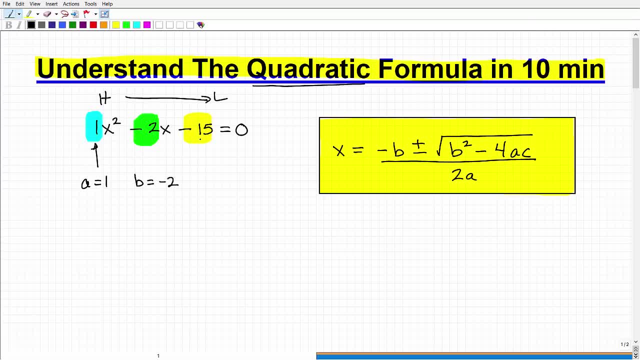 So b is equal to negative 2.. And then the number itself is c, So c is equal to negative 15.. And you make sure you get those signs in there as well, whether they're positive or negative. So a general form to use a quadratic formula is a x squared. 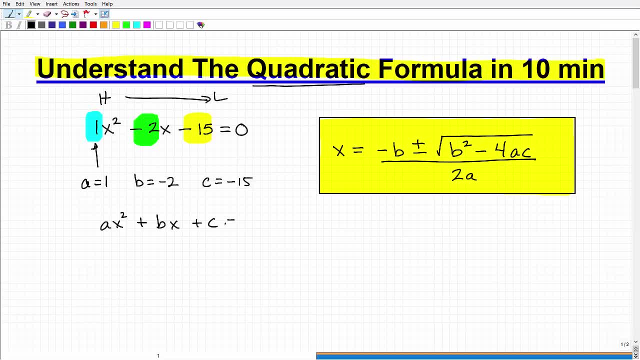 plus bx plus c is equal to zero. So if you have a polynomial equation in its general form, the number in front of the x is a. the number in front of the- I'm sorry, the number in front of the x squared is a. 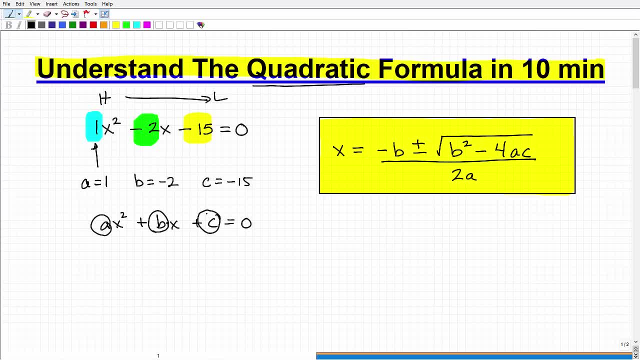 the number in front of the x is b, and then the number out here by itself is c. Okay, So you can see that in this particular example. Okay, So, now that we have our values for these variables, a, b and c, 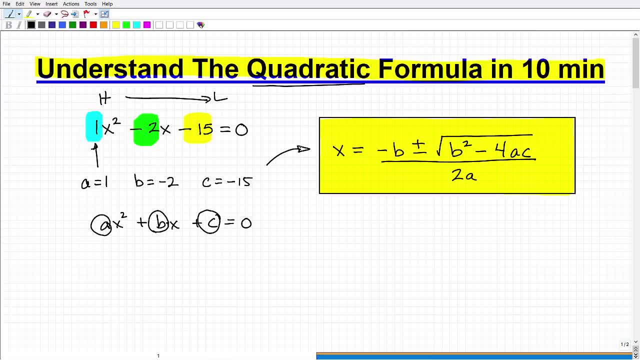 we simply plug them into the quadratic formula And we're going to go ahead and find our two solutions. Now, a lot of you out there probably already understand this part. As a math teacher of you know decades, I've seen thousands, tens of thousands of problems. 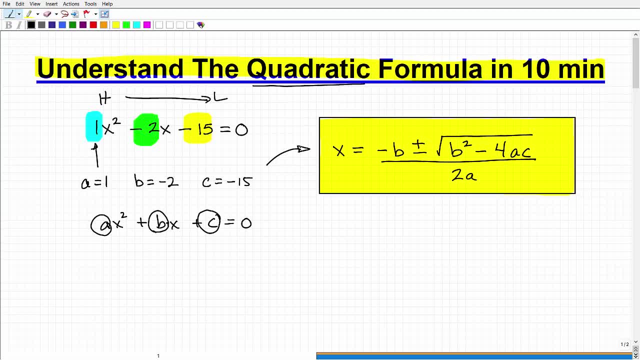 students, you know, doing the quadratic formula, you pick up on common mistakes, common trends. So I'm going to really try to point them out to you so you don't make these common errors. So let's go ahead and continue on with this problem. 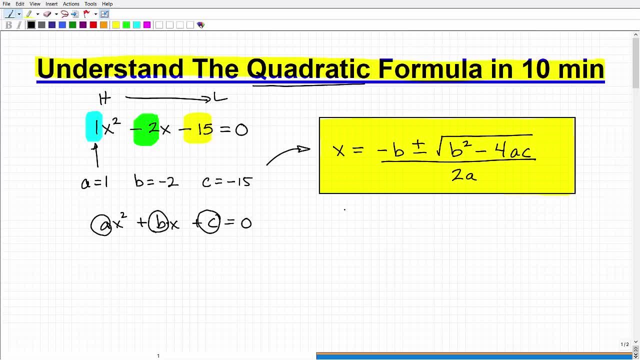 and I'll point out these common- you know trends here in a second. All right. So when we plug things in to the quadratic formula, we've got to be super careful. So this is like the first place where students make a mistake. 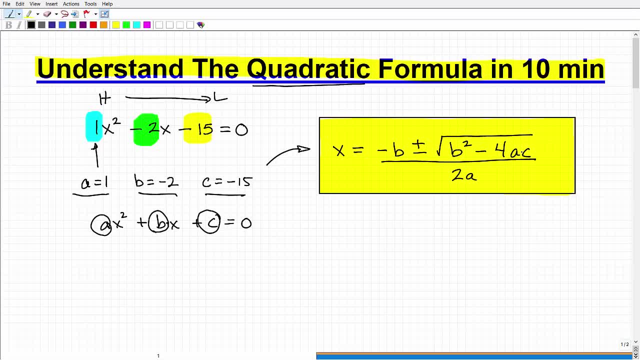 They understand the a, b, c part, but they plug things in not correctly into the formula. But let's go ahead and do it now. So we have x is equal to minus b, So b is negative 2.. Here I'll go ahead and put little boxes around them. 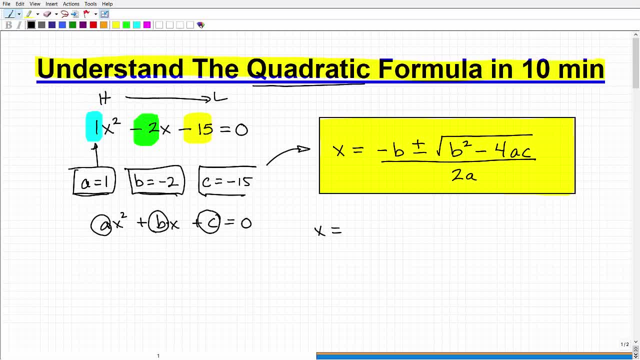 Okay, a is equal to 1,, b is equal to negative 2, and c is equal to negative 15.. And specifically where students mess up is when you have negative signs with these values. they get confused here, So the best thing to do is to use parentheses. 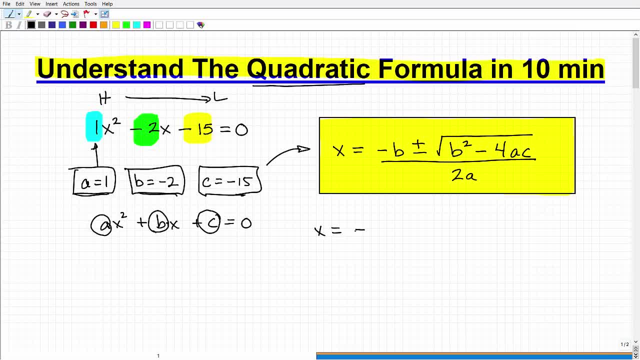 So x is equal to minus b, So just put the minus sign there and b is equal to negative 2. So you need to put parentheses negative 2. Your b value is negative 2. So plug that in. So anytime you're replacing this variable with the value. 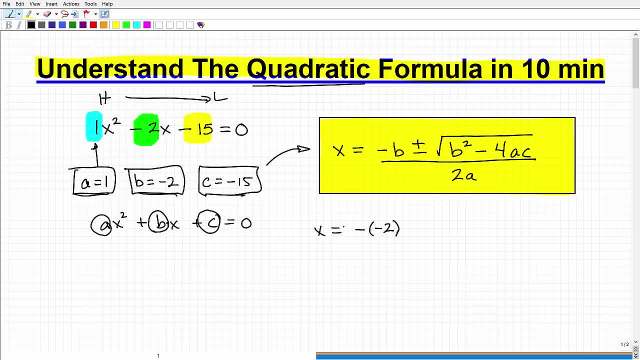 use parentheses And that's just a good general rule to follow in algebra, okay, when you're evaluating expressions. So we have minus b, okay. So that's going to be minus and minus 2, plus or minus, And I'll get into what the plus or minus means as we work through this problem. 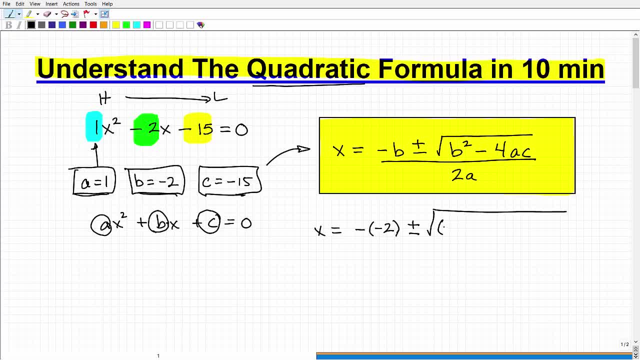 The square root of b squared again, it's going to be minus 2.. That's b squared minus 4 times a. a here is 1, right, I'm just following the formula- and c is negative 15.. 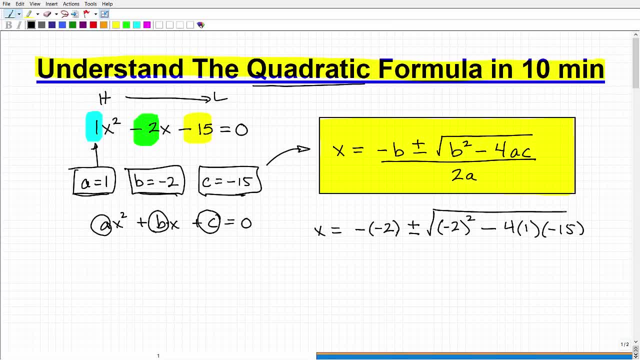 So I'm using parentheses to plug in these values And notice, my square root goes all the way over the b squared minus 4ac part And this is all going to be divided, one big long fraction bar by 2a, So that's going to be 2 times the value of a and that is 1 in this case. 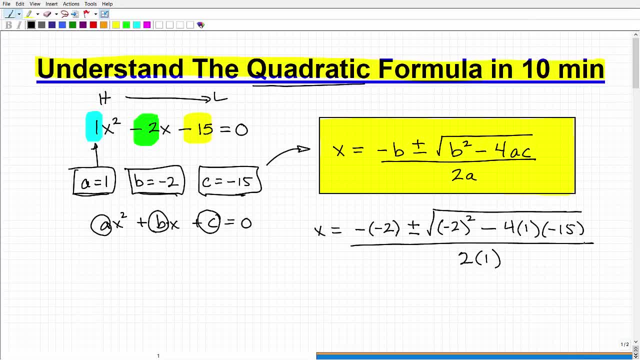 All right, once you've done this, you want to double check your work. Okay, A lot of students. they'll plug in the wrong values and then they'll do that part correctly. They'll do it as if they plugged in, like they're doing another problem. 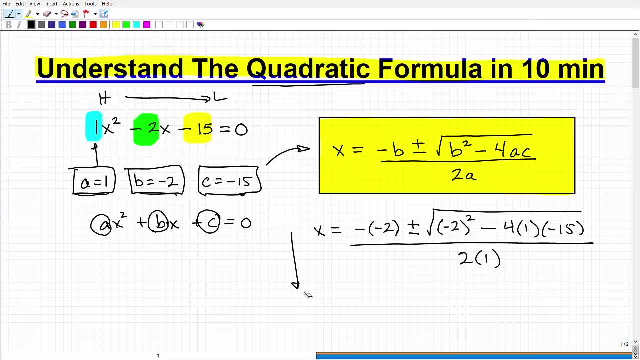 They did it perfectly. The only problem is they plugged in the wrong value, So don't start simplifying the math here until you double check, okay. So in other words, just kind of quickly look. okay, is that b, b squared? 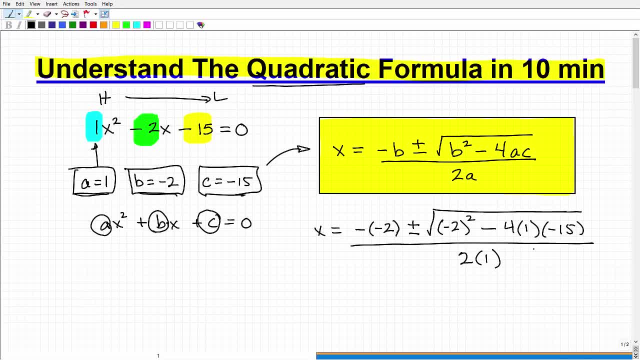 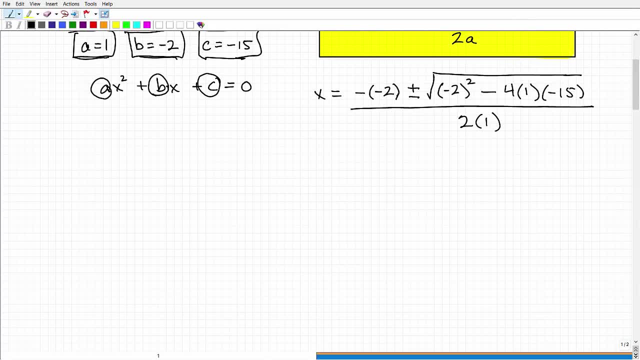 Just double check that you plugged everything in correctly. If you you know, once you've done that and you feel good about it, now we're going to go ahead and do the math here. Okay, so what I'm going to do? I'm just going to grab this and kind of scoot this into the center. 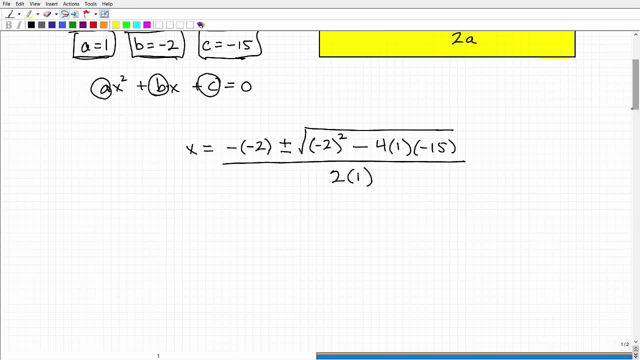 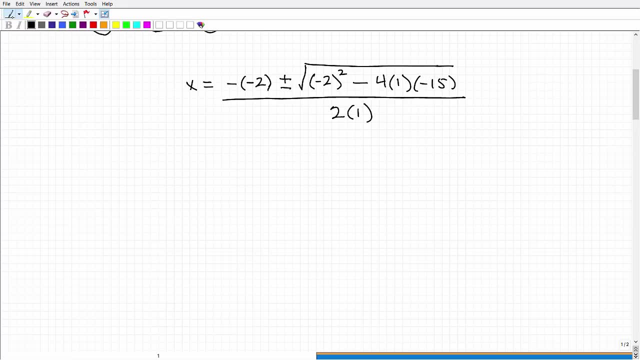 so we can work a little bit better. All right now. this is basically now an order of operations problem. You need to go nice and slow, step by step, and you should be writing the steps down. Don't try to calculate all of this in one step, okay. 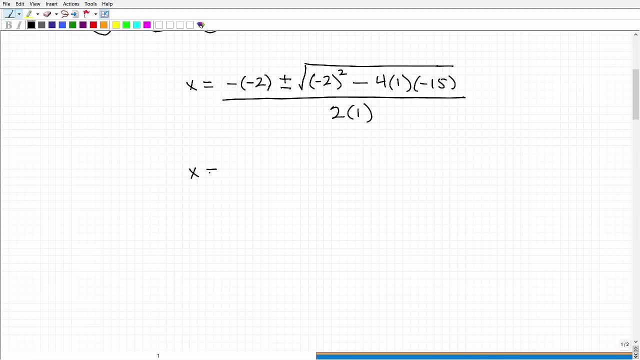 So I'll go ahead and show you. So you're going to just kind of rewrite this: x equals minus, 2 is what. That's. positive 2, right. The opposite of negative 2 is 2.. So that's going to be 2 plus or minus, and let me just stop here. 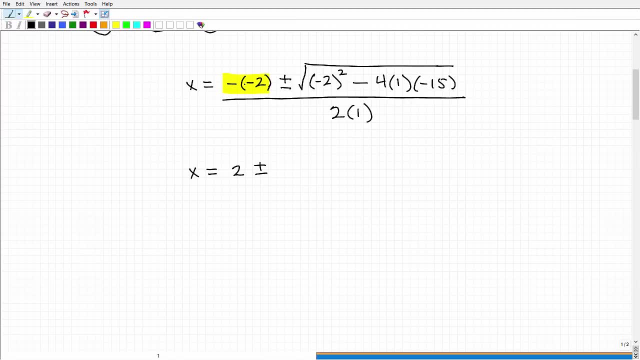 If you didn't understand this, that means you need to go back and work on your positive negative number rules, real number rules, okay, So again, you know, as I'm doing this, if you don't understand something, you're probably having trouble with the quadratic formula. 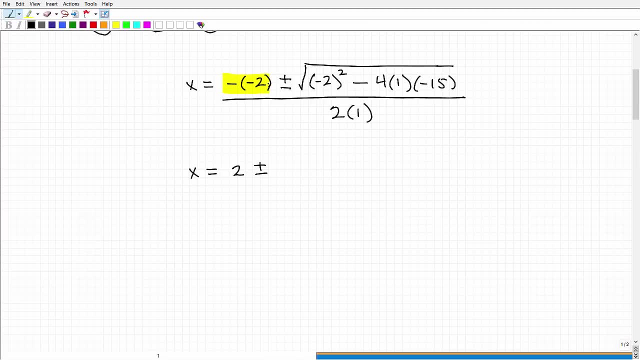 not because of the formula itself. It's because you need to review your, you know, positive, negative, number rules or fractions or whatnot. okay, So let's continue on. So negative of negative 2 is positive 2 plus or minus the square root. 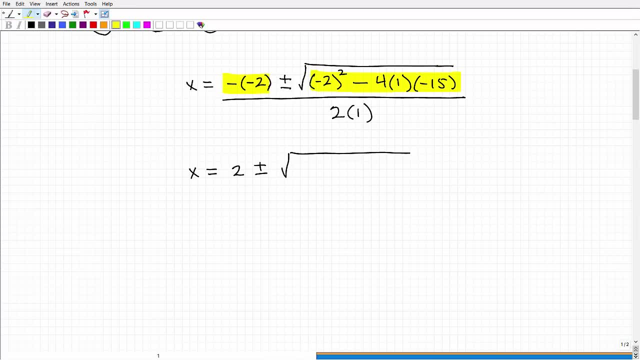 and just kind of work this down one at a time. okay, So negative 2 parentheses squared means this: That's a negative 2.. Negative 2 squared means negative 2 times negative 2.. So that is going to be equal to a positive 4, all right. 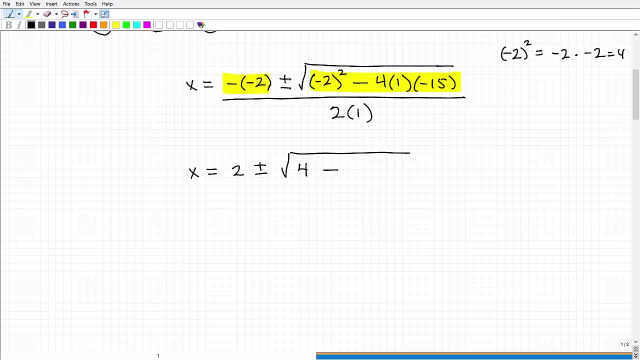 So I'm going to write that right here: minus 4.. So I'm going to write that right here: minus 4 times 1, okay, times a negative 15.. So I'm just kind of writing this out like this: okay. 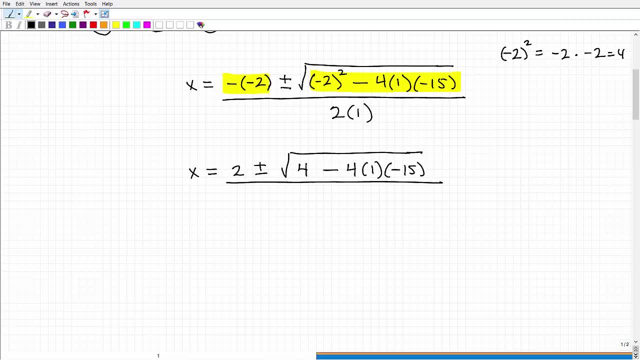 I haven't done any more steps here. All over 2 times 1, and that's 2.. So I'm just kind of simplifying: one or two steps at most per line that I'm writing. okay, Now let's continue to move forward. 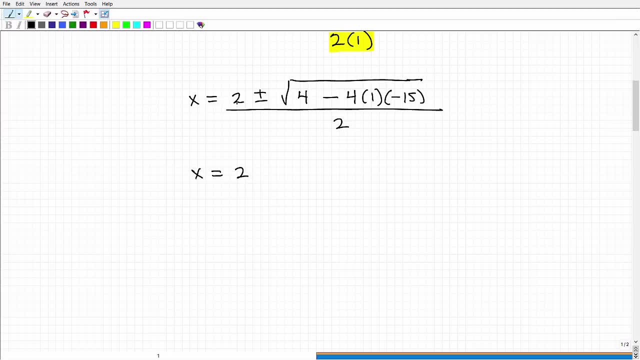 So x equals 2.. I'm just rewriting this again. okay, There's nothing here I can do yet, But I have to rewrite it: 2 plus or minus the square root of 4.. Now, what I'm going to focus on is this part, right here. 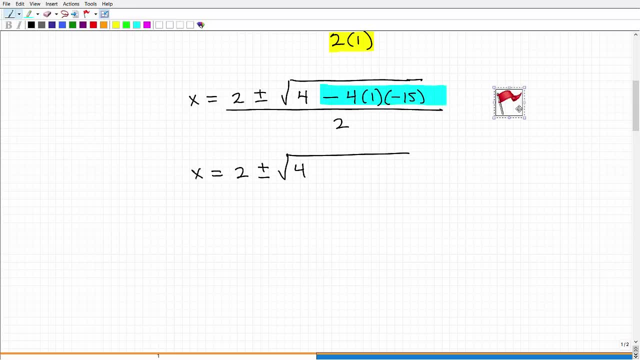 And this is another very common place where students mess up, okay. So I'm going to give you a little technique, a little tip here on how to avoid this. Students- well, they'll confuse the signs, They'll get this wrong, okay. 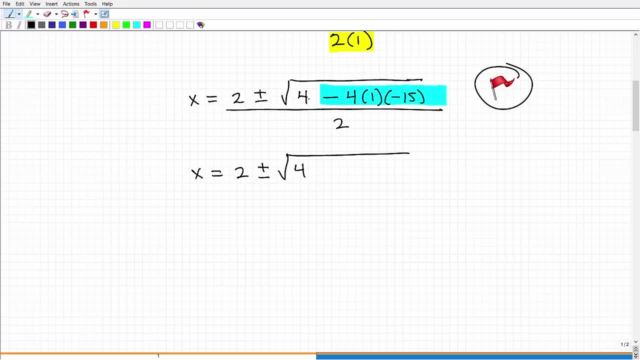 Again, many, many students. They do get these problems wrong. get them wrong. You know they make them an error right here. So 4 minus, it's going to be 4 minus 4ac, or 4 times 1 times negative 15.. 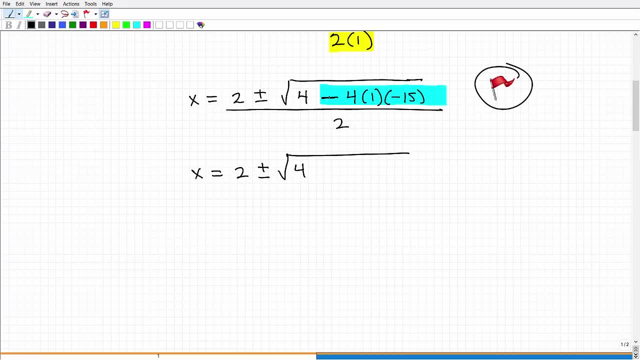 This minus sign. do yourself a favor, Turn it into a plus negative, because this is really a negative 4, a plus negative 4.. So b squared minus 4ac. This is the part in our formula It really means, Or you can think of it as: b squared plus a negative 4 times a times c. okay, 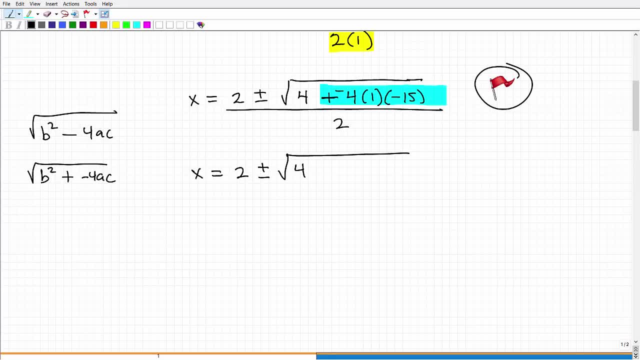 And students. invariably, you know, they get this problem wrong. They more than 50% of the time. they make an error right here, okay, So what I always suggest to students if you're making that mistake, if you get confused. 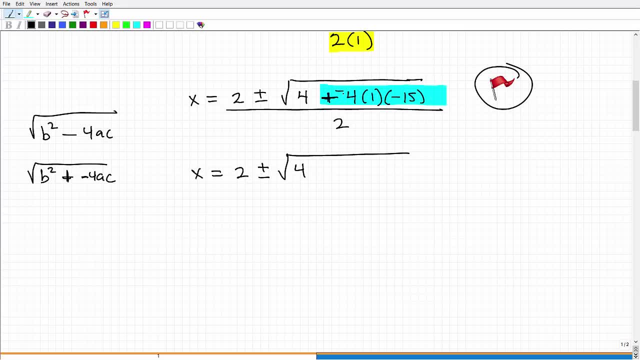 just turn this into a plus negative 4.. So now we have plus negative 4 times, 1 times negative 15.. And just really kind of focus on what's going on here. So now I have 4 plus. let me kind of back up here. 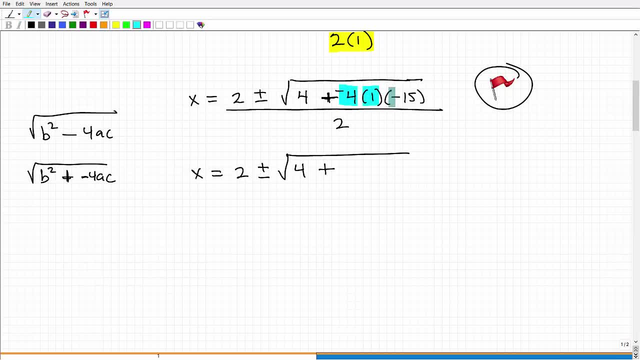 And we have to figure out what negative 4 times 1 times negative 15 is. So this is going to be a negative times a positive, which is negative. So our negative times a negative, this whole thing is going to be positive here. 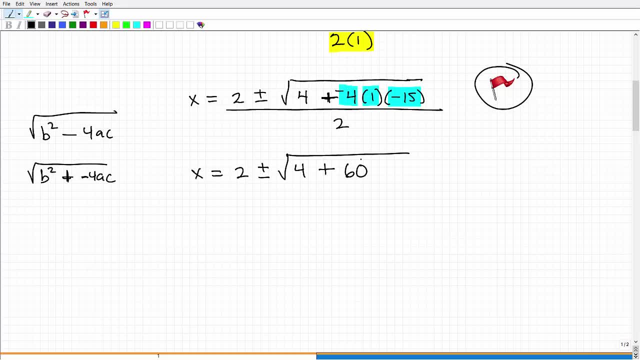 And it's going to be a positive 60, okay, Now that's going to be all over 2, okay, Which was 2 times 1, so it's just 2.. So now we're kind of getting there. Things are kind of. 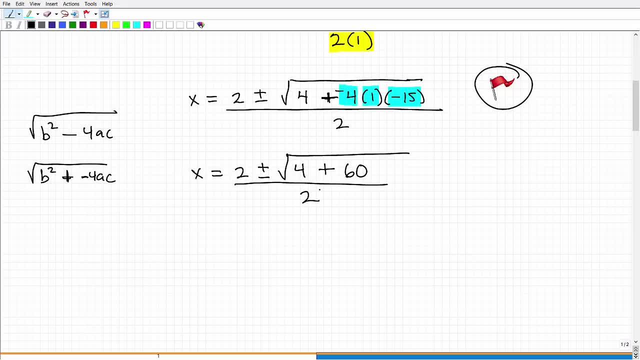 We're kind of past some of the more common mistakes, The big things here that students make a mistake on is they plug in incorrectly, okay, Because they get confused with the negative numbers And then they also make a mistake with the b squared minus 4ac, okay. 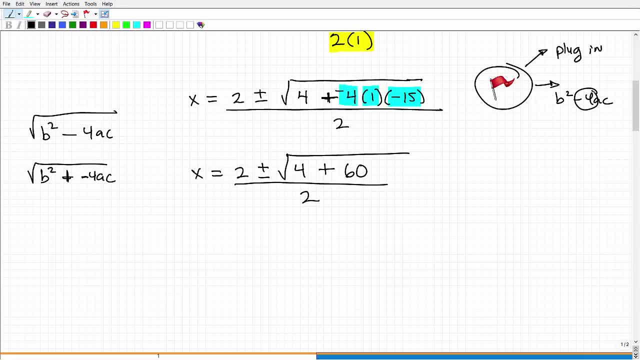 This part right here. all right Now, let's continue to move on here. Now it kind of works sideways. This is equivalent to 2 plus Or minus the square root of 4 plus 60. And that's 64 all over 2.. 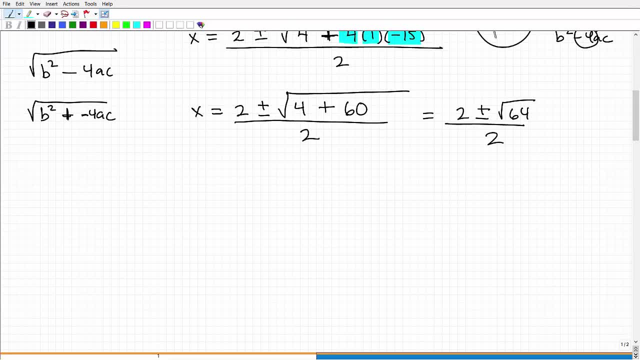 And this problem is going to be finished up here pretty quickly. Let me scoot this down. All right, Now I'm going to put it here. All right, so x equals 2 plus or minus the square root of 64.. 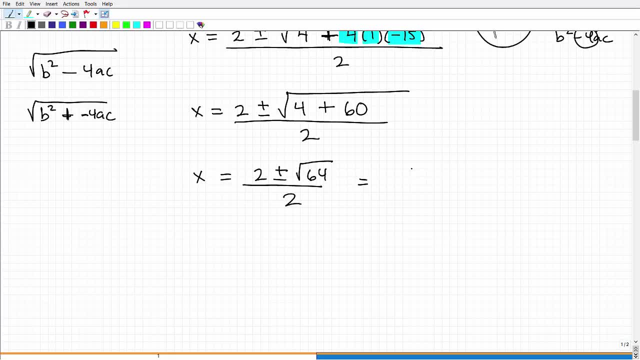 So the square root of 64 is 8,. okay, It's technically plus or minus 8.. And that's why you have the plus or minus here. okay, So 2, the square root of 64 is 8, plus or minus 8 all over 2.. 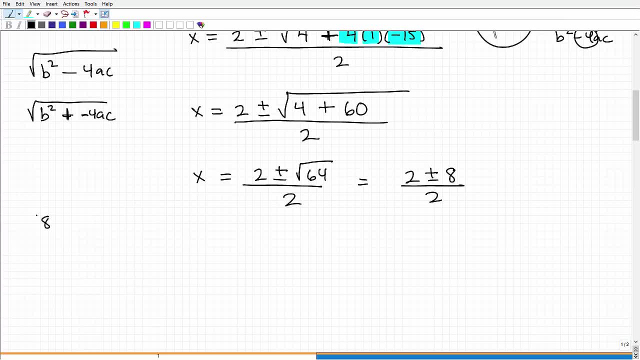 Think about it: 64 is 8.. Positive 8 times a positive 8 is 64.. However, negative 8 times negative 8 is also a positive 64. So your answer is both plus or minus. So the square root of 64 is: 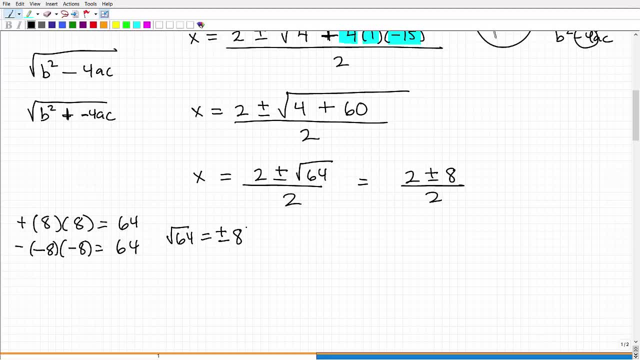 It's both a positive and negative 8. Now, being at the square root of any real number, positive real number is going to be plus or minus. It's already built into the formula. That's why you have that plus or minus there. okay. 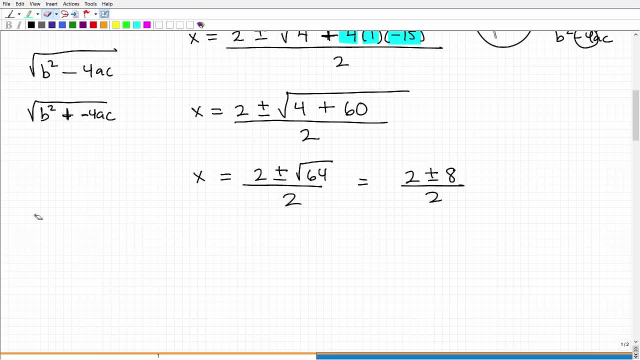 So I'm going to erase that. I just wanted to point that out to you. Remember, when you're doing math, like, let's say, the quadratic formula, if you really understand how to do one problem, then you should be okay doing multiple problems. 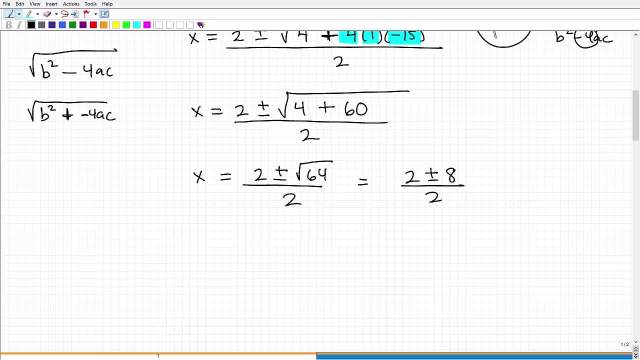 So I'm really pointing out things here, nice and slow, so you can really kind of master this, And of course we want to try to Do this in 10 minutes and I'm sure I'm probably a little bit over that right now. 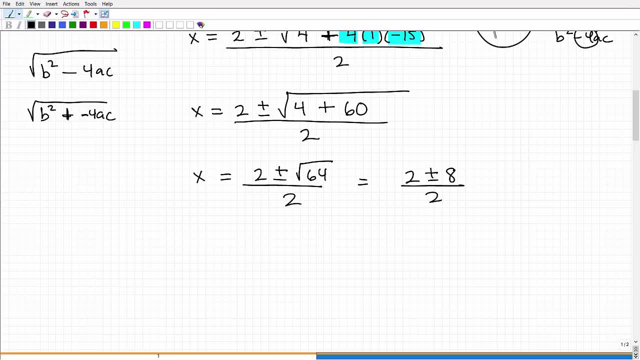 but who cares? By the time you get done watching this video, you'll be a quadratic equations formula expert. All right, let's finish this thing up. So we've got 2 plus or minus 8 over 2.. So what do we do at this point? 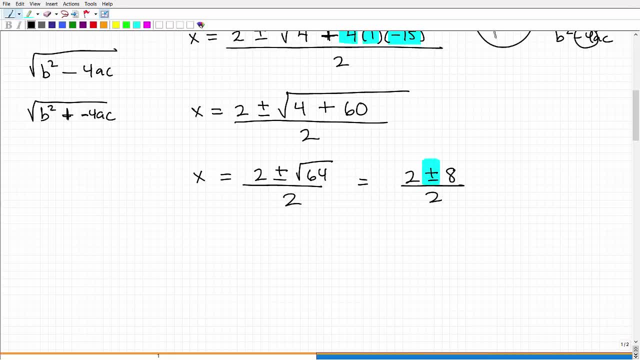 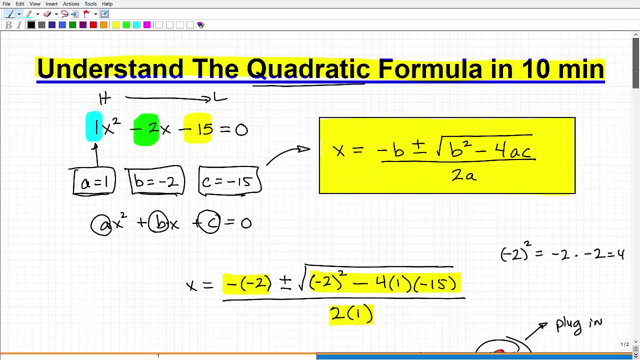 Well, this plus or minus here is critical. This is how we're going to get our two solutions. Remember- let me kind of go up here real quick- When I talked about the theory of polynomials x squared. there's two solutions. 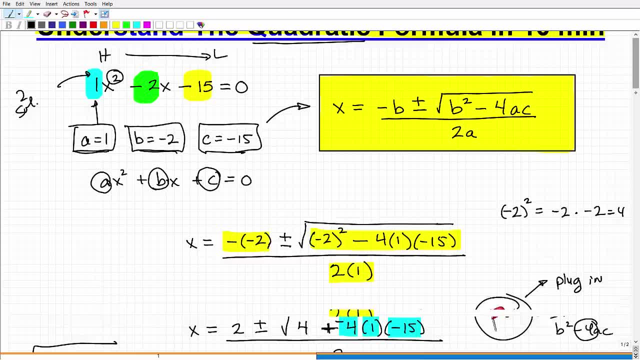 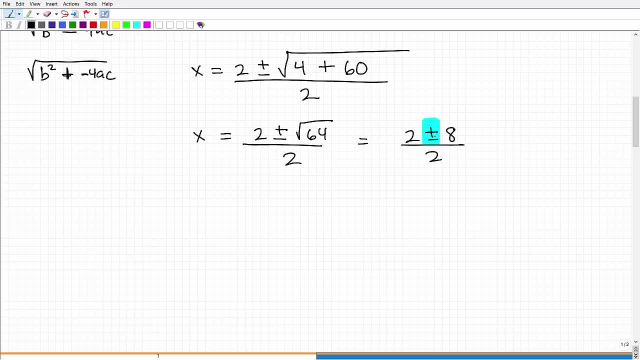 You always get two answers with the quadratic formula: Always, always, always. If you don't, you're doing something wrong. Now, this plus or minus is how you're going to get it, okay. So what this means, and we want to break it out this way- 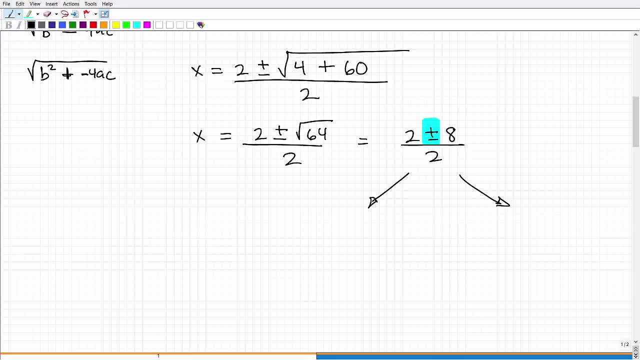 is the following: We want to write this as 2 plus 8.. We'll do the plus here, 2 plus 8 over 2, and then we'll do the 2 minus 8 here- Okay, Over 2.. 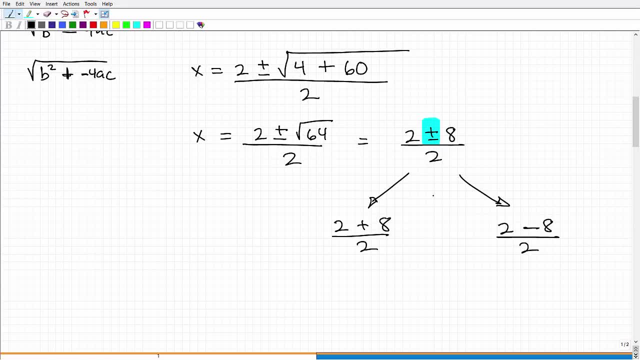 So we have a plus 8 and a minus 8.. We're not going to write it all out. Typically we'll just write this as plus or minus 8.. But at the end of this problem you have to write out. 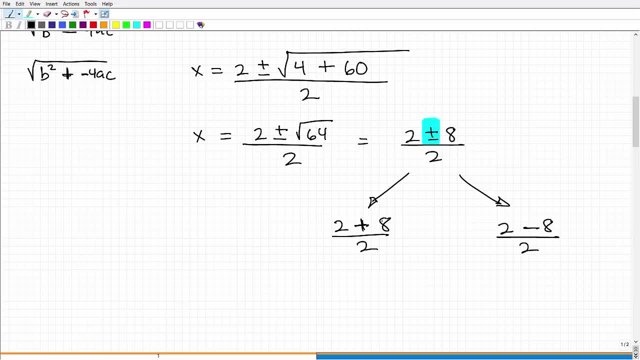 you actually have to do each calculation separately, okay, And this is how you're going to get your two answers. So you have: 2 plus 8 is 10,, obviously divided by 2, and 10 divided by 2 is 5, okay. 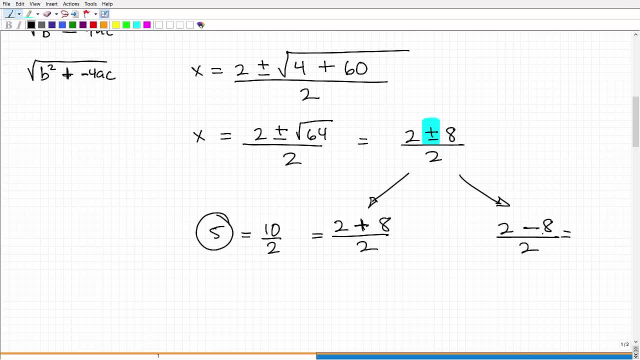 So that is one solution, all right. And then over here I have: 2 minus 8 is negative 6 divided by 2, and negative 6 divided by 2 is negative 3.. And that's my second solution, okay. 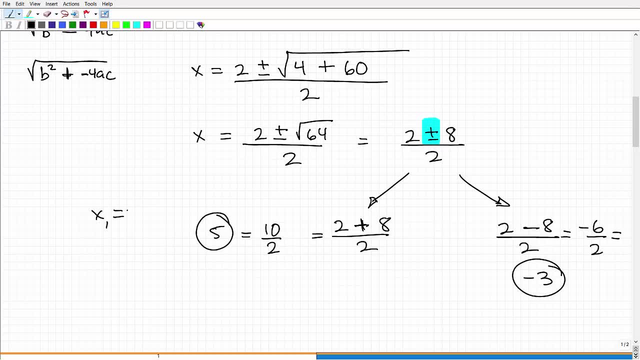 Sometimes you'll see this written as x1 being 5 and x2 being negative. 3, okay, So you can even write this out this way: x1 and x2, all right. So that's the notation. Sometimes it varies a little. 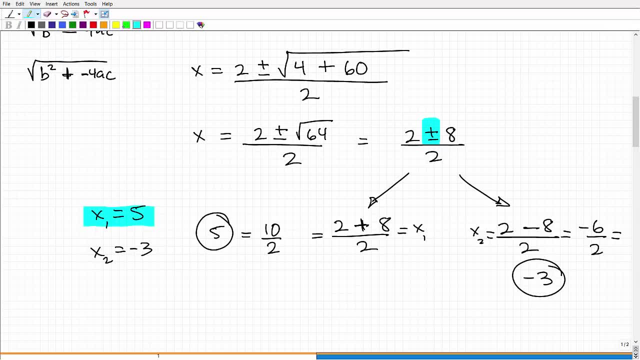 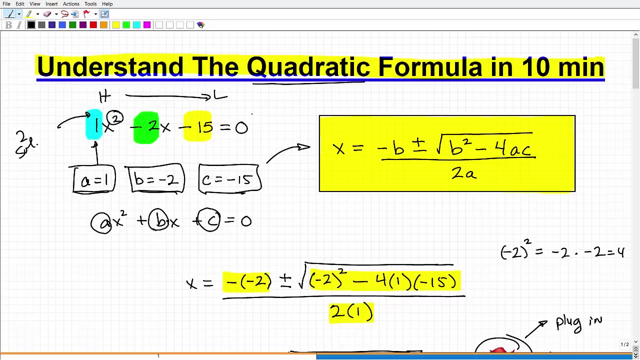 But here's the bottom line. You have two solutions to this quadratic equation, okay, So hopefully you understood this. Let's quickly, quickly, go back up here and review again, all right, Just really fast. So here is a polynomial equation. 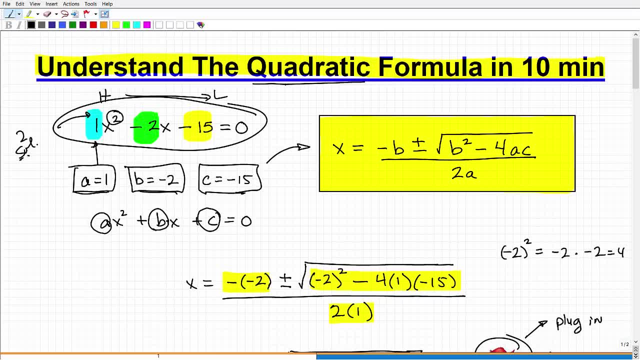 It's quadratic because the highest power is 2.. It also means that you'll always have two solutions. Once you have this guy written in standard form- highest to lowest power- we can assign values to the variables a, b and c. okay. 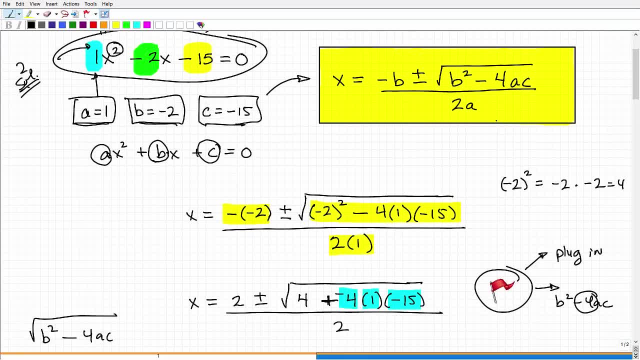 So that's the first step. Now, obviously, you need to have the quadratic formula handy. I wouldn't suggest you memorize it right off the bat when you're learning this, but you should commit this to memory. The first place that you really have to concentrate is plugging in correctly. 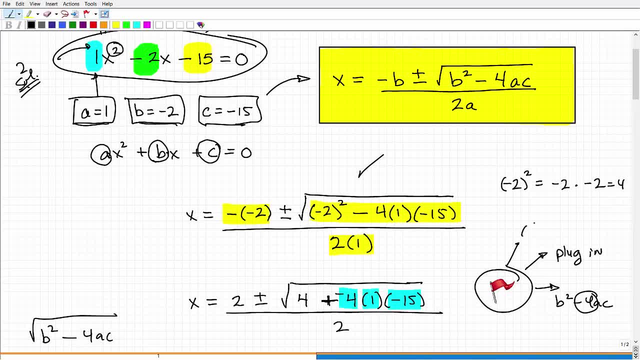 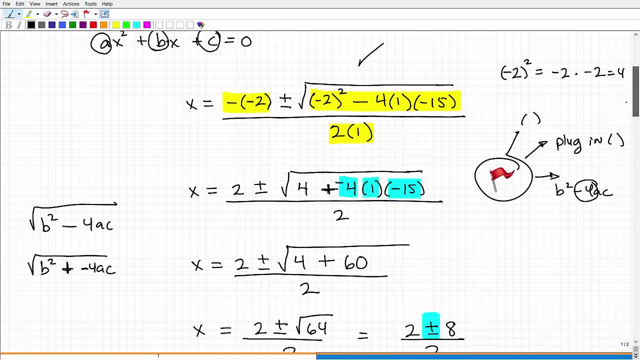 Use parentheses. okay. So we actually will put parentheses here, but you have to plug in using parentheses and then you double check That you plugged everything in correctly before you continue on. So before you do all this other work, make sure you plugged in correctly, okay. 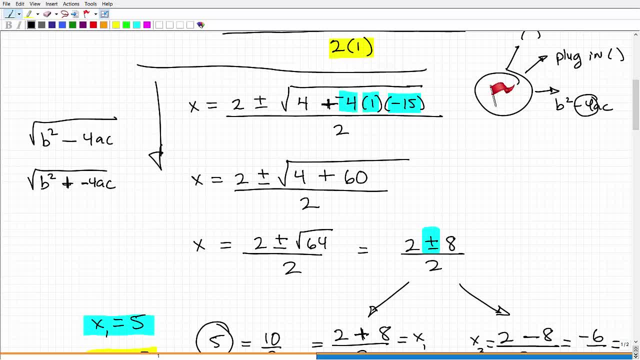 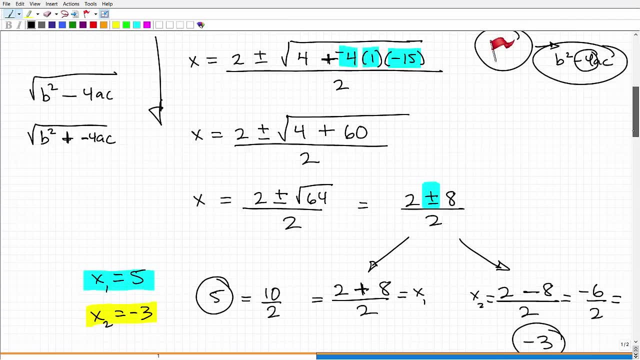 As you kind of start simplifying and you do it step by step. watch the b squared minus 4ac part- Big big place where students mess up And then just kind of work through your calculations and then be mindful that the plus or minus part. 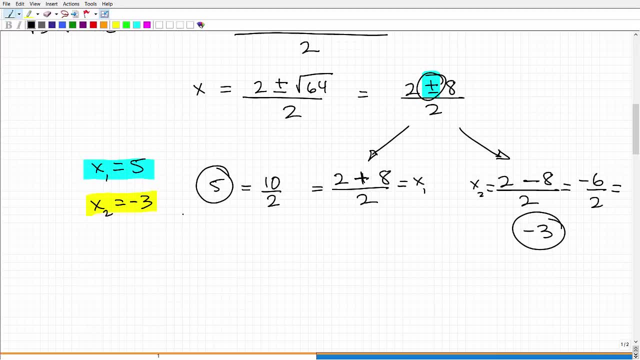 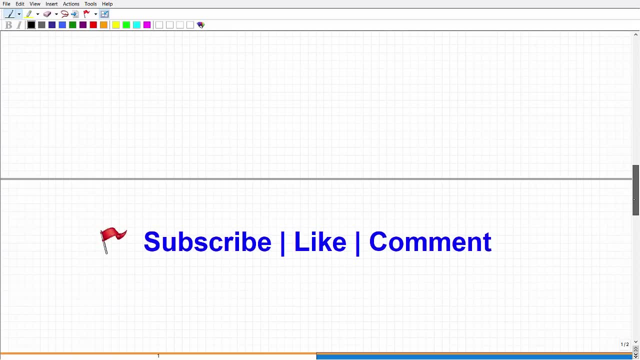 is where you're going to get your two separate solutions. Okay, so that's it for this video. You know, of course, there's much more complicated problems with the quadratic formula. It's a big topic in mathematics and algebra, You know you can be using. 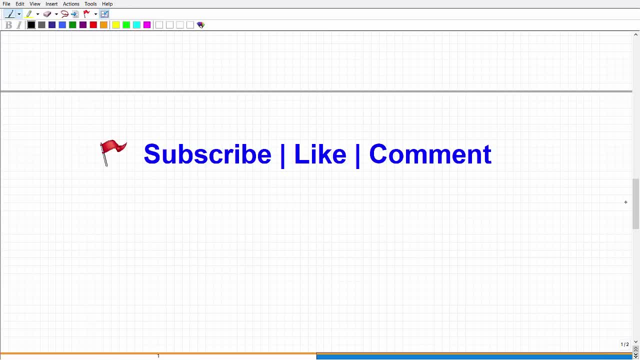 By the way, you can use the quadratic formula with fractions and decimals, and then there's positive and negative roots and then imaginary roots. Probably some of you out there are like: oh, what happens? You know, this is a much deeper topic. 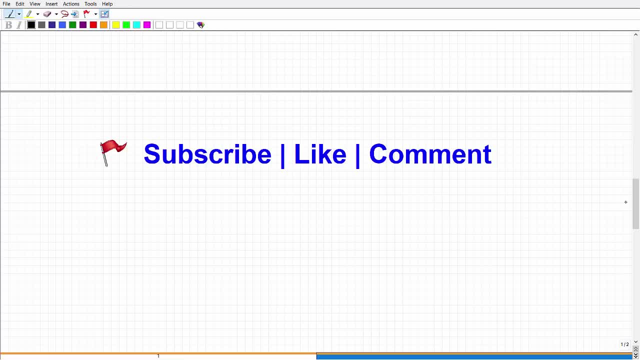 The whole point of this video was just to get you to apply the quadratic formula. Okay, now the theory of polynomials. that's more expansive And hopefully you'll subscribe, because I have a lot of stuff on my channel about that, about the quadratic equations, polynomials, etc. 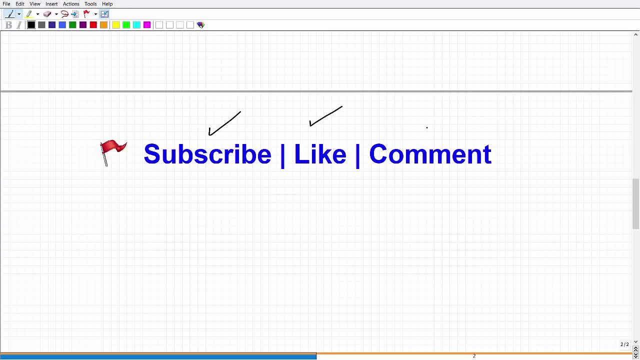 And if you know this video helped you out, maybe you want to consider giving it a thumbs up and leave me some feedback. I try to read as many comments as possible so I can figure out what kind of videos that you could best serve the community out there. 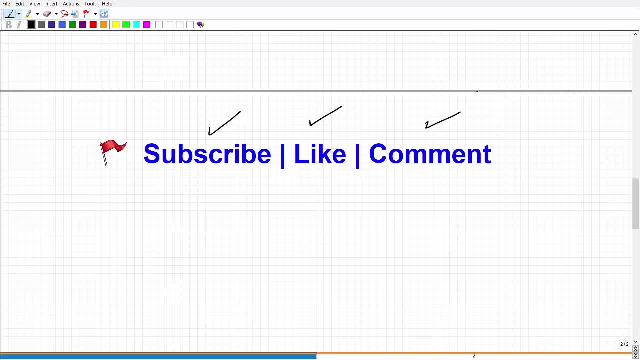 But anyways, appreciate your time and I wish you all the best. Take care.